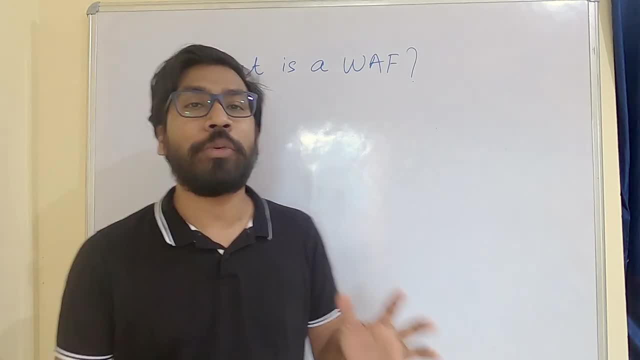 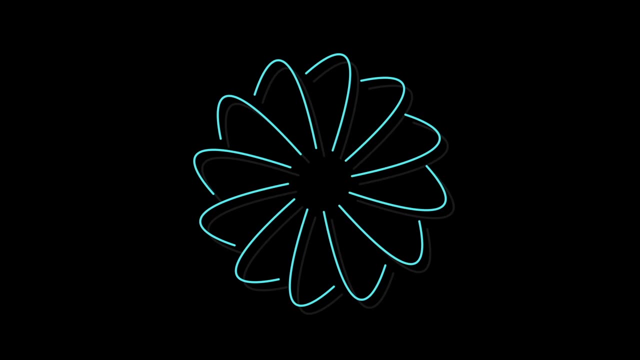 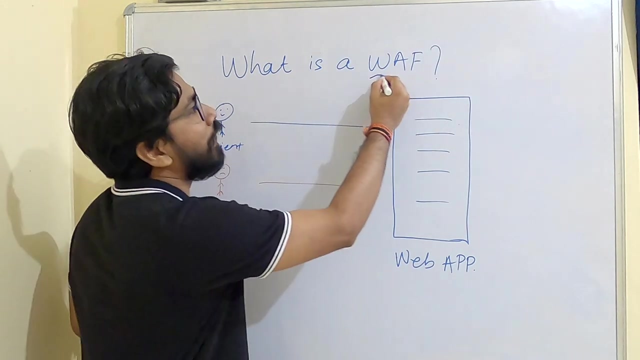 Hello friends, I am Trilochan. I hope you are safe and healthy. Today we will discuss what is web application firewall. So, without any further delay, let's move forward. So let's understand what is web application firewall. So this is your web application. 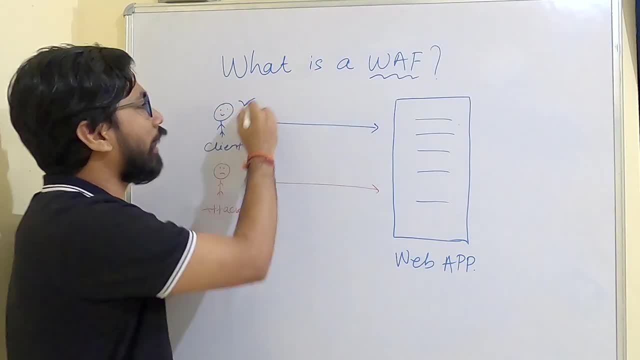 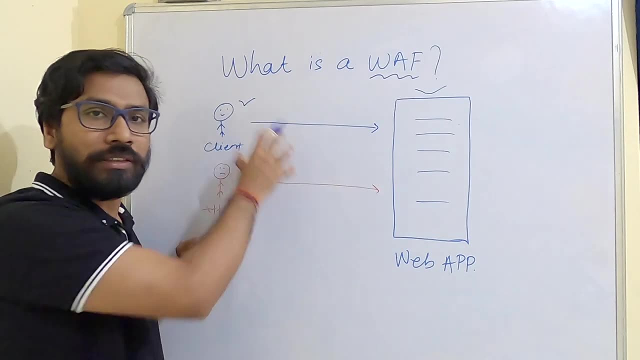 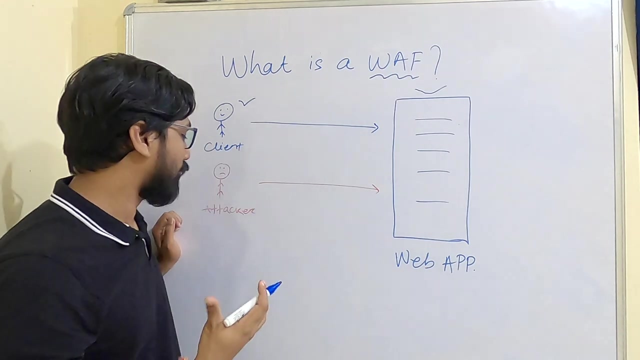 and you have some clients. These are the clients and these are the web applications, and they are using or accessing your web applications and enjoying your services. So what? some clients are there, those have bad intentions and those are called attackers. So now the question is: 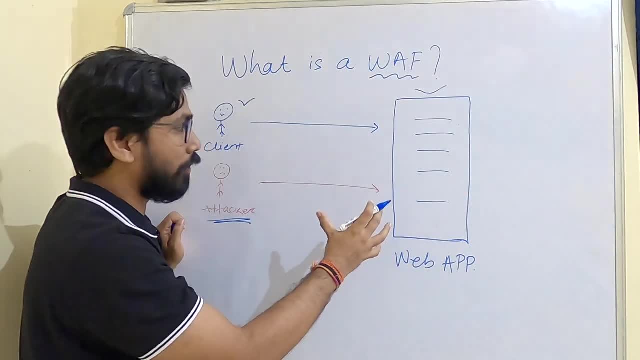 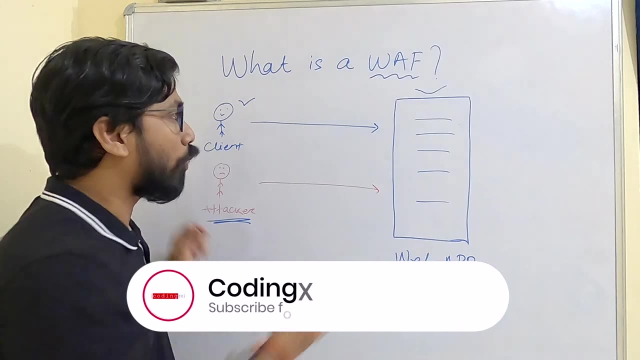 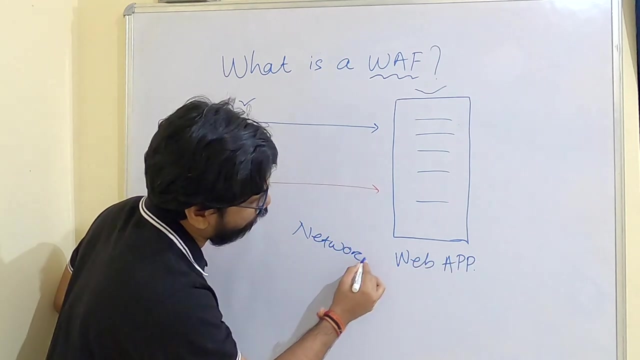 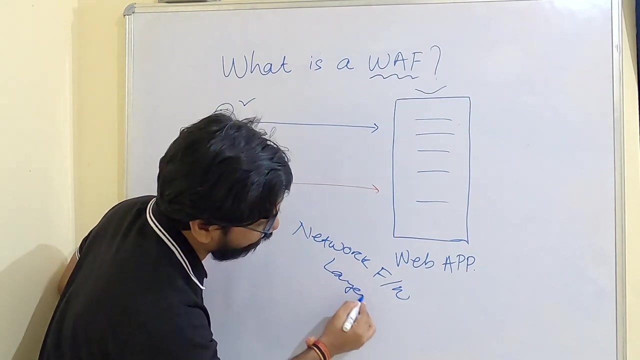 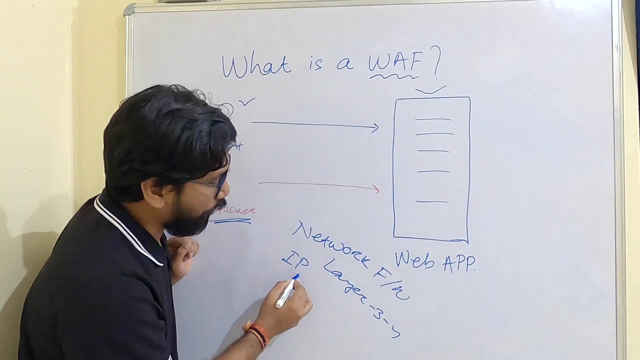 how do you protect your web applications from these attackers? So it's a typical and standard way to protect your web application. We deploy network firewall And this is happening layer 3 and 4. And through network firewall we can protect IP or filter. you can say filter or monitor. The bad IP is through the network firewall. 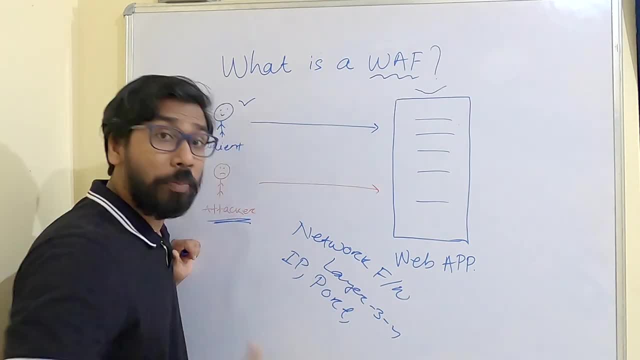 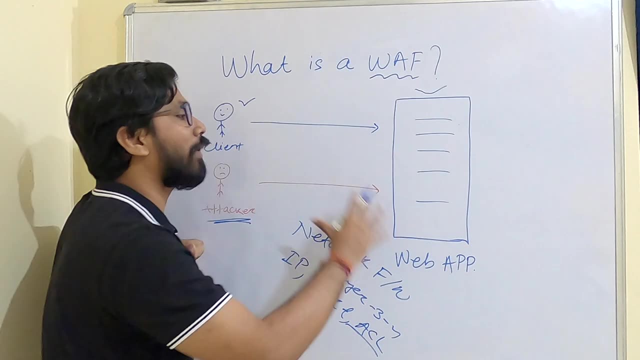 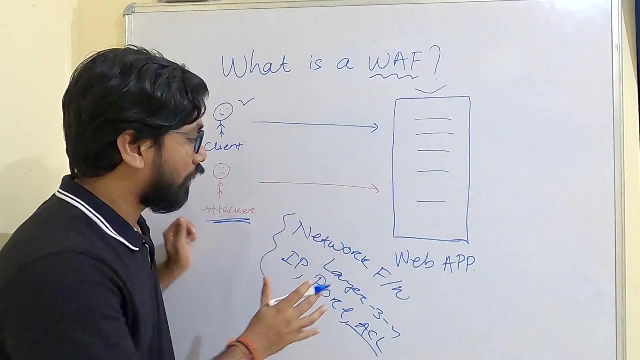 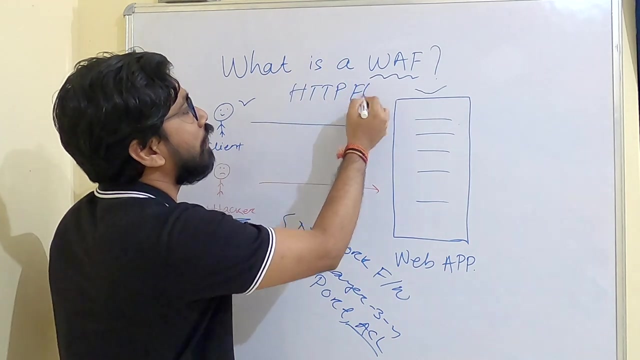 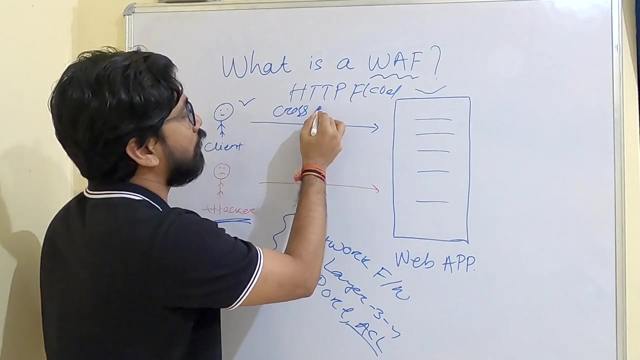 and we can restrict particular port and we can make some list of access control like CL, So that our web application protect by this network firewall. But some attacks are there, like you can. I can give an example: HTTP flood and cross-site scripting. cross-site scripting. 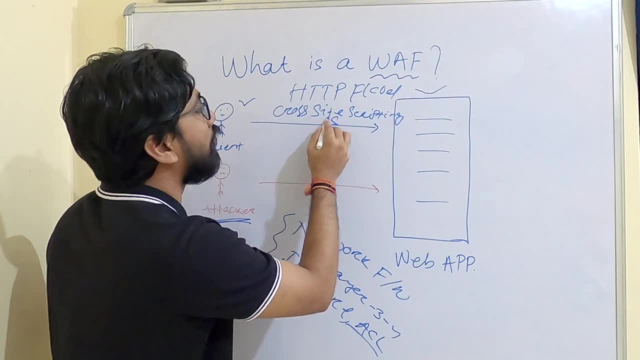 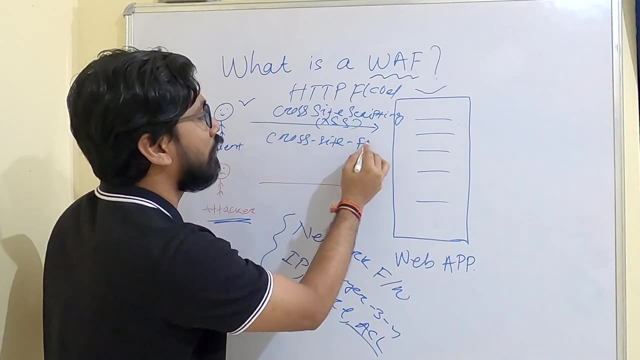 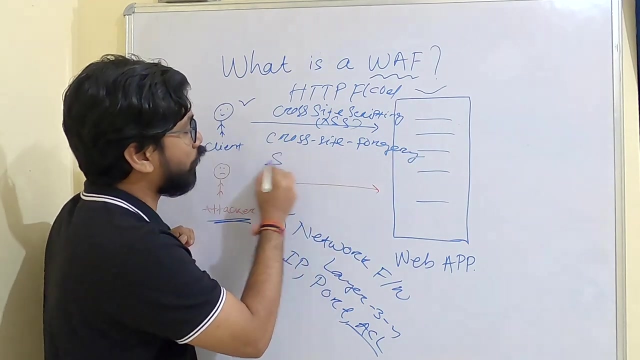 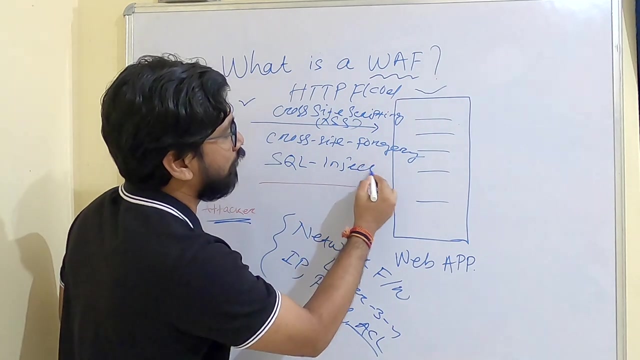 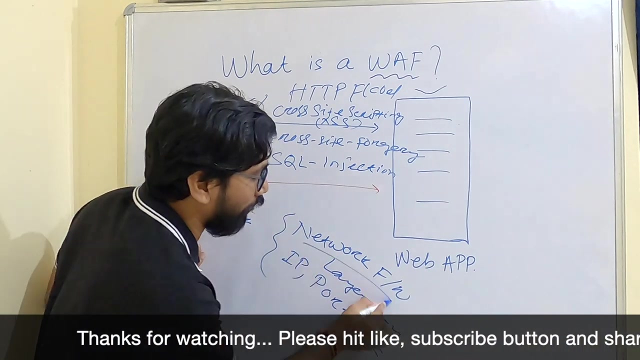 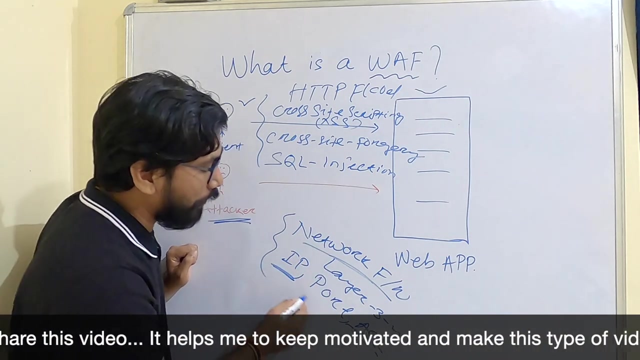 scripting and you, I think you heard of XSS and cross-site Perjury, and the most common attack is SQL injection. This attack usually happens And these attacks are not designed for the network firewall. attacks are easily passed through this network firewall and they have valid IP, valid port.